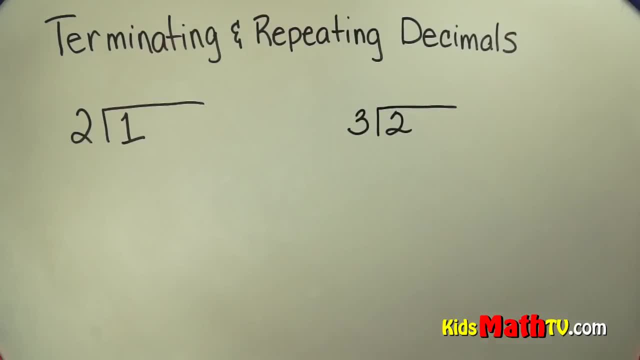 In this lesson, we will learn about terminating and repeating decimals. Here we have two into one or one divided by two. In order to do this, we can put a decimal place and some zeros, and I can put as many zeros as I want. I'll just start with two there. Bring my decimals. 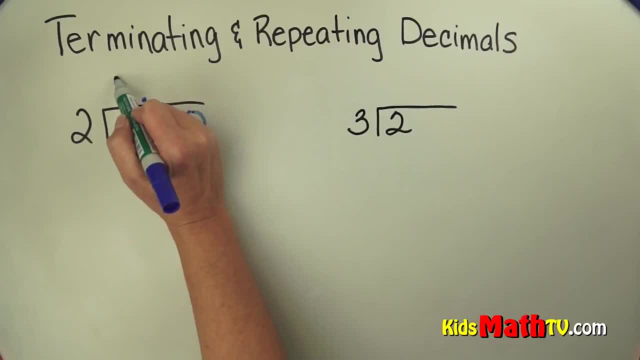 straight up. How many twos are in one? There are zero. How many twos are in ten? Well, there are five. Five times two is ten Subtract, and it comes out even So our answer is zero and five tens or one half. So one divided by two is one half. That makes sense Here. 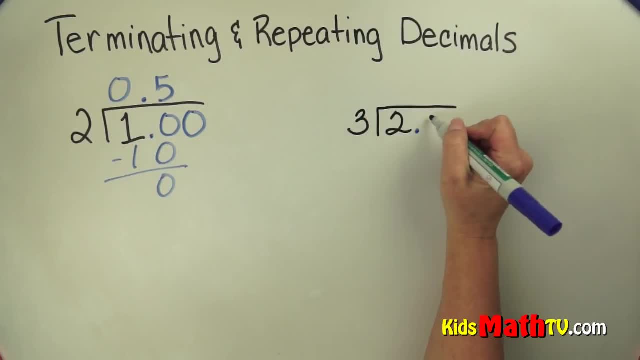 I have two divided by three. So again I'll put my decimal and a couple zeros and then I start my decimal straight up. And how many threes are in two? There are none. How many threes are in one? There are none. How many threes are in two? There are none. How many? 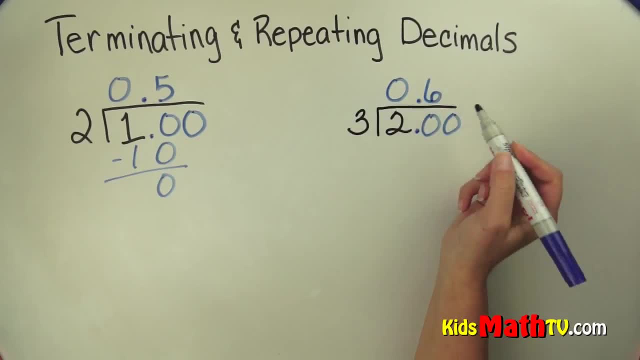 threes are in one? There are none. How many threes are in two? There are none. How many threes are in twenty? Well, three times six is eighteen, That's as close as I'll get. So eighteen. And then I subtract, and when I subtract I get two. So then I bring down. 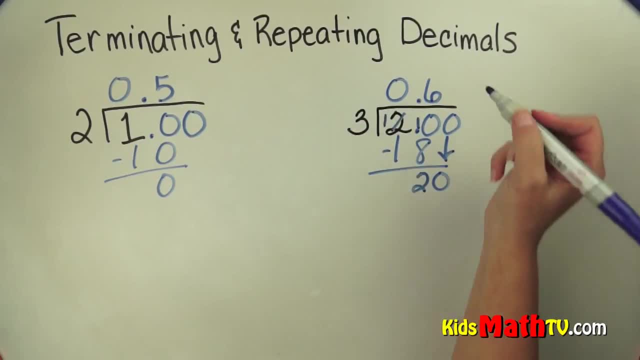 a zero. Now how many threes are in twenty? Well, six, Six times three is eighteen Subtract. and again, I'm going to get twenty. and I will keep going like this forever and ever, and ever. So we can round this. Well, let's go one more time here. 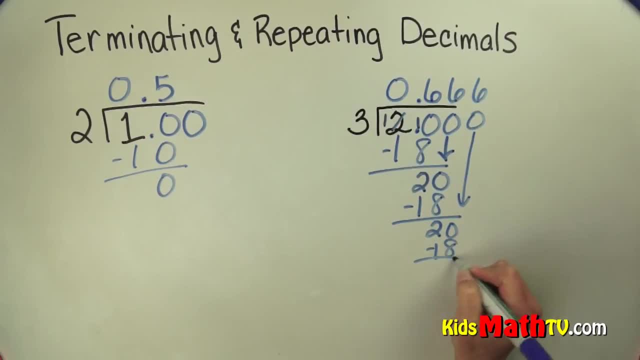 This would be another six Eighteen subtract zero. So I'm going to actually round this. I can round it to either zero and six, with the line over it- Okay, And that tells me that it's repeating. Or I can round it to the nearest hundredths And let's see This. 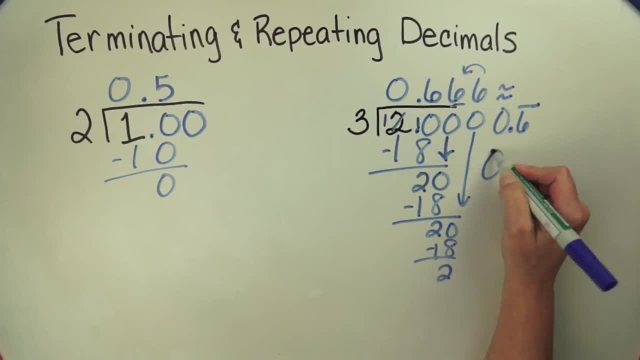 is the hundredths place, That six tells that to go up one And I can make that zero and sixty seven hundredths Either way, And that's the end of this lesson on terminating and repeating decimals.